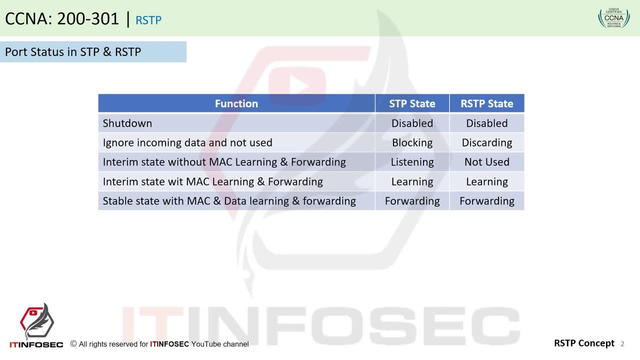 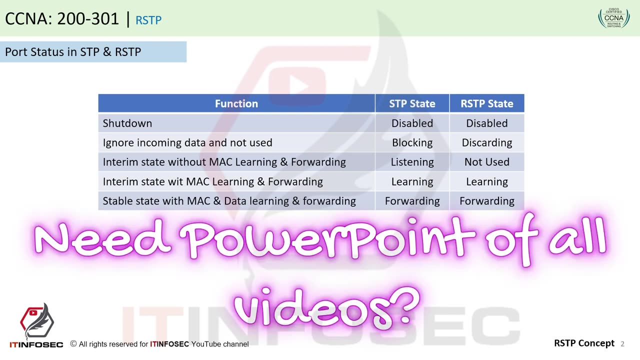 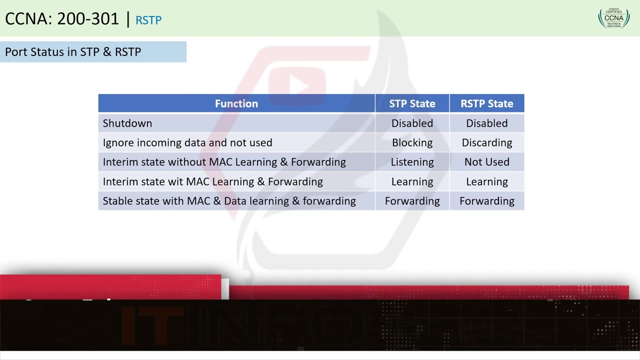 have a very comprehensive lab about switching and we will examine all switching technologies from vlan to bpdu in a complete lab at once. now let's go to this issue. if you remember, we said that scp was started automatically between the switches to prevent loops in the network. well, a switch was chosen as the root switch, and the status of that. 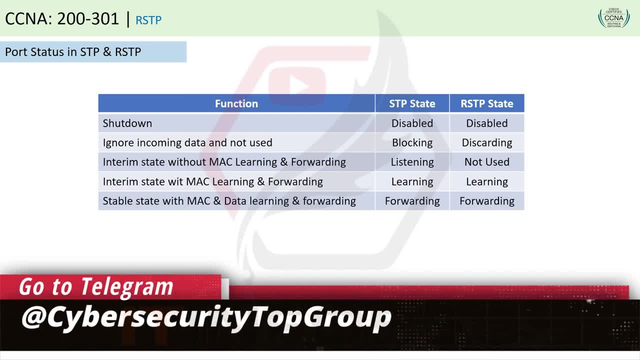 of all ports between on all switches was determined accordingly. you can see that we have a very comprehensive lab about switching and we will examine all switching technologies, from vlan to bpd, in a complete lab at once. now let's go to this issue. if you remember, we said that scp was started automatically between the switches to prevent loops in the network. well, a switch was chosen as the root switch and the status of that of all ports between on all switches was determined accordingly. 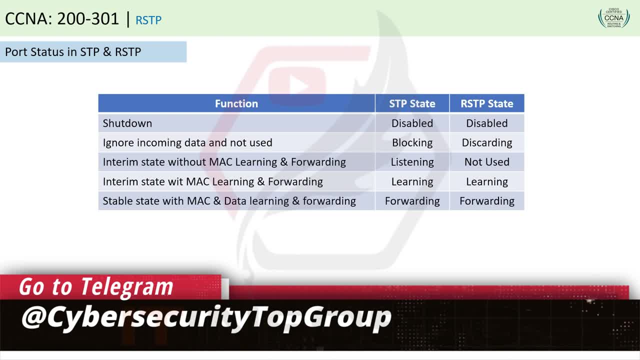 well, a switch was chosen as the root switch and the status of that of all ports between on all switches was determined accordingly. now, if the root switch was changed for some reason, the port that was blocked in other in order to prevent the, the loop would be changed and another port would be would be blocked, okay. 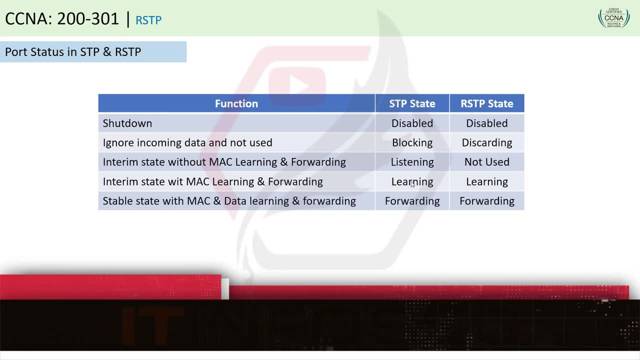 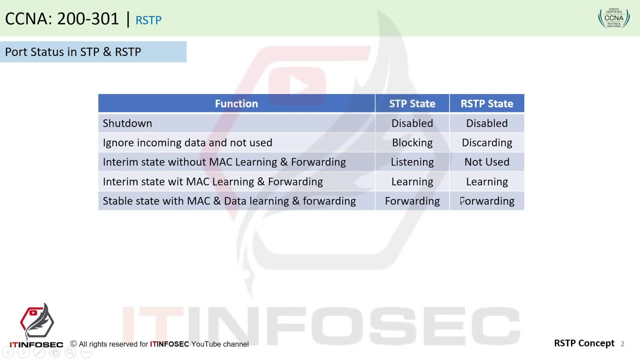 this table shows the difference between stp port states versus rstp port states and this discuss about this. but what is rstp? rstp is rapid, is rapid spanning tree. it is the fastest spanning tree or faster than the stp. if you shut down the port by manually, by shutdown command, in stp state the port will shown as disabled and in rstp shown. 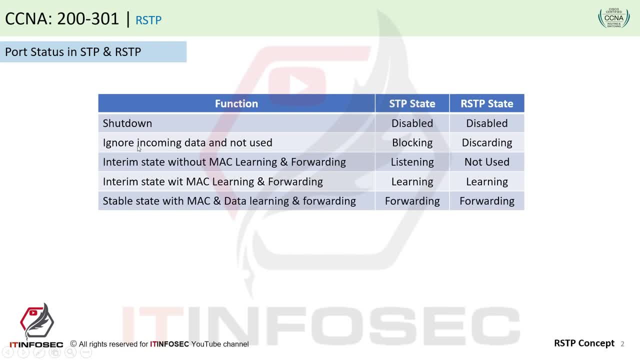 as disabled as well. if the port function or port status ignoring coming data are not used in stp, the port function or port status ignoring coming data are not used in stp state will shown as blocking and in rstp shown as discarding. in the if- uh, if it is in interim state without mac learning and 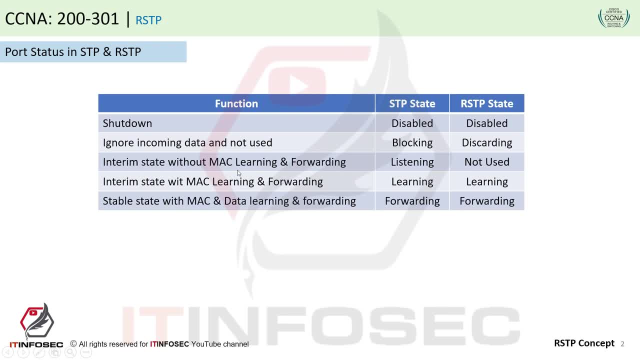 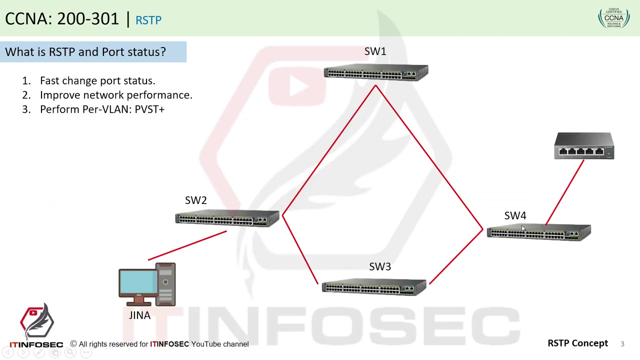 forwarding but not disable or block interim state without mac learning, not listening. we don't make learning and forwarding in stp state shown as listening and rstp doesn't have like this item. And if port status is an interim state with MAC learning and MAC or data forwarding. MAC forwarding- sorry it is- means learning in STP and in RSTP shown as learning as well And in a stable state with MAC learning and data forwarding in STP forwarding and in RSTP shown as forwarding. 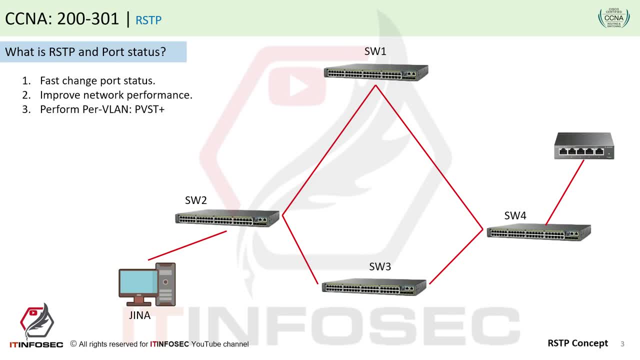 Now this is our network. Imagine we have SW1, SW2, SW3, SW4, one computer connected to SW2 and one hub switch connected to SW4. If we run the STP between the switches, if we have the RSTP, the connection between two switches, known as point to point, 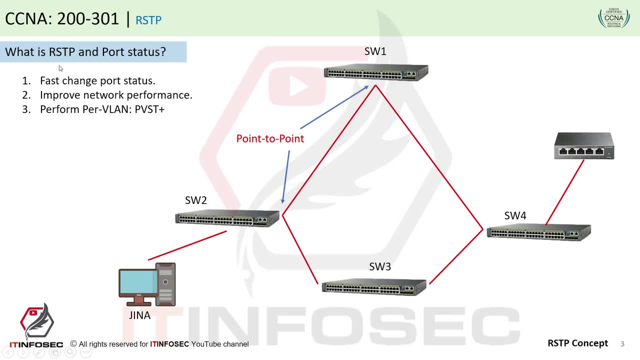 These are the port status when we have or when we started RSTP And if we connected. if we have a network connected from SW4 or from the switch to the hub to the another device which is hub switch, it's known as shared port. 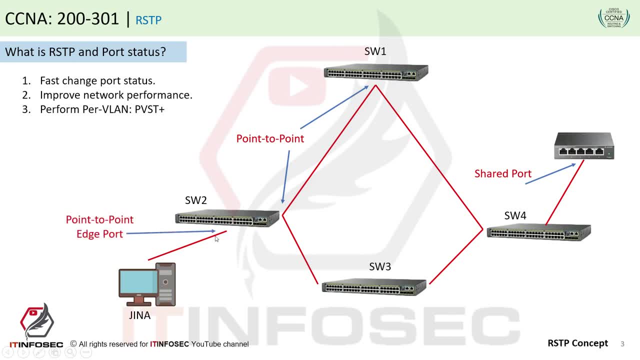 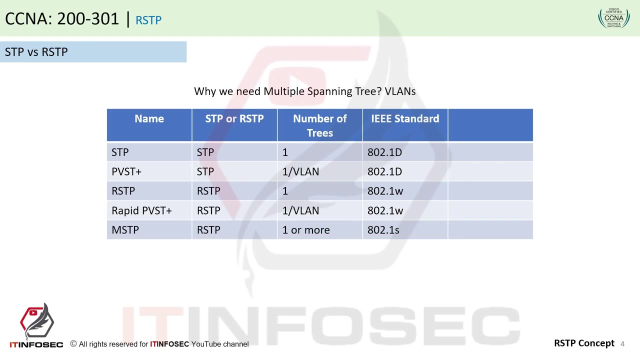 And we have connect. if we have connected the computer to the switch, it's known as point to point edge port, because it is the end of the network. it is the edge and the network will not continue after this. But the main question is why we need multiple spanning tree. 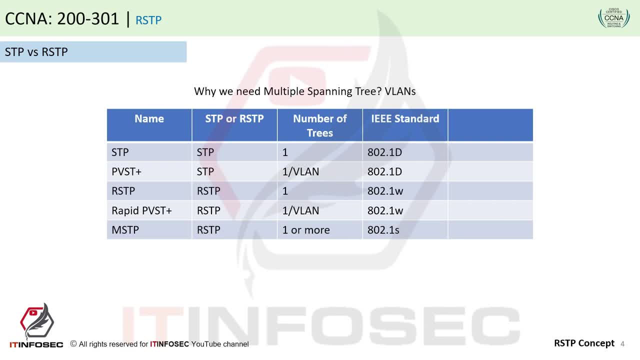 And the response is VLANs. Maybe you need to have some VLANs, for example, one VLAN for sales department, one VLAN for human resources department, one VLAN for finance department, and so on, And maybe you need to put some switches based on each department, based on each port. 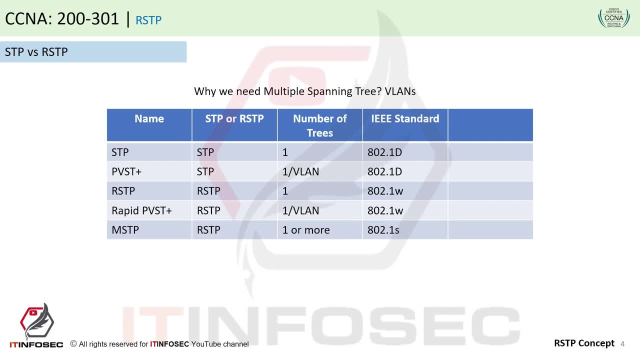 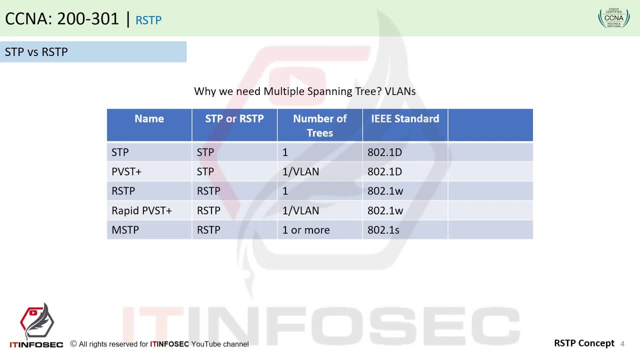 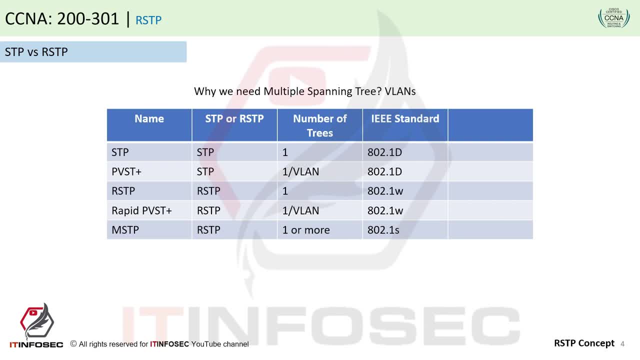 And maybe, based on your security policy, based on your networking needed configuration, maybe need one switch in one department to be a root switch and that switch in another VLAN for another department. It's a not required to be a root switch and another switch will require to be a root. So if you have 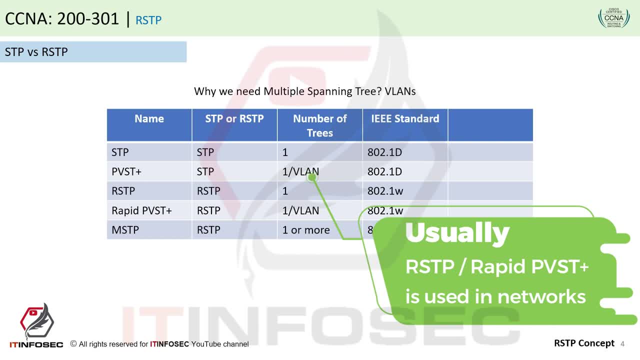 multiple VLANs. the result is maybe you need per VLAN, one switch, for example, be a root and per another VLAN another switch may be a root. But the SDP is a standard protocol for S53 performing that's known as a standard 802.1d, and after that the Cisco created. 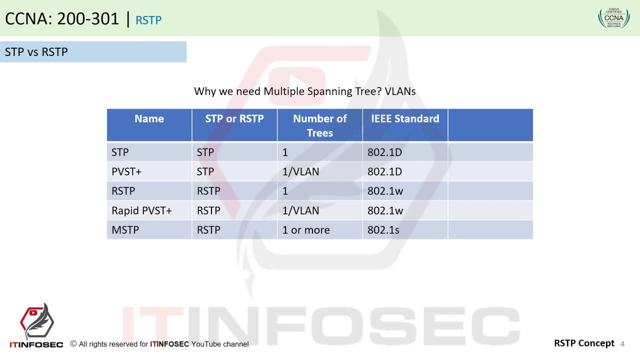 Cisco proprietary SDP protocol, or per VLAN spine tree. that's known as per VLAN spine tree plus or PVST plus. Again, after implementing and introducing RSTP, RSTP or 802.1w protocol, in 2001 Cisco created another proprietary protocol. 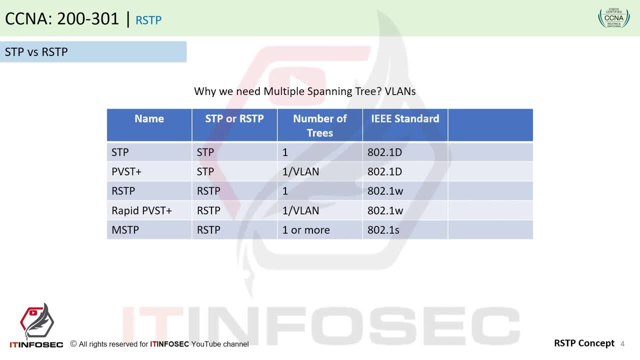 that's known as rapid per VLAN, spine tree plus or RPVST plus, sorry, Okay, so this table show about these protocols: SDP- it is SDP based. and number of trees: number of trees for preventing loop between the switches: it is X13, and known as and a known 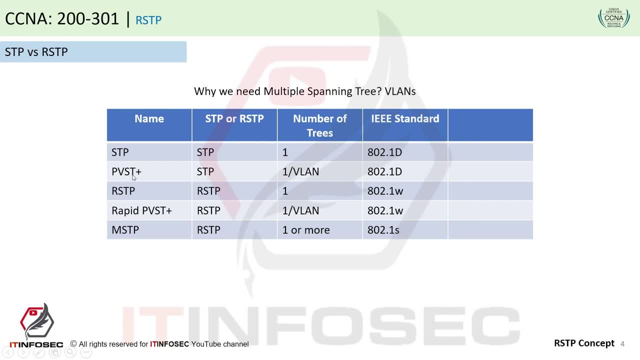 under a standard 802.. 1 D per VLAN securities, re plus or previous C plus is categorized under SDP and one per媽n no more trees per room and one and 802.1 D protocol. if we perform an internet RSTP it's categorized under RSTP and number of trees just. 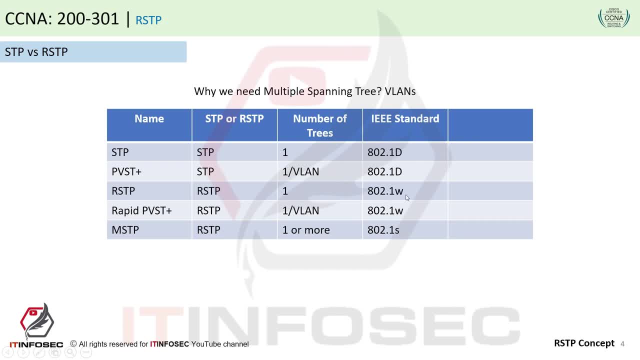 just one categorized under 8, under 2.1 w protocol. if we have rstp, our pvst plus rapid pvst plus, it is categorized under rstp per one per vlan. if you have, for example, five vlan, you have five separate uh and anti-loop uh, rpvst plus implementation and maybe you have five. 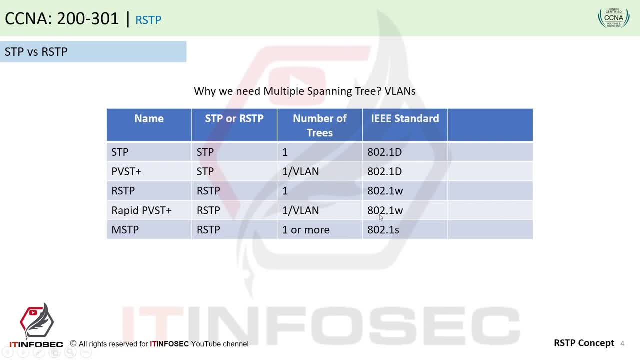 different root switches and 8 under 2.1 w and multiple spanning tree or mstp. that allows definition of many instances, for example, multiple spanning tree instance that chosen by the network design but not required, one per wheel and definitely maybe one or maybe more than one, and categorized under: 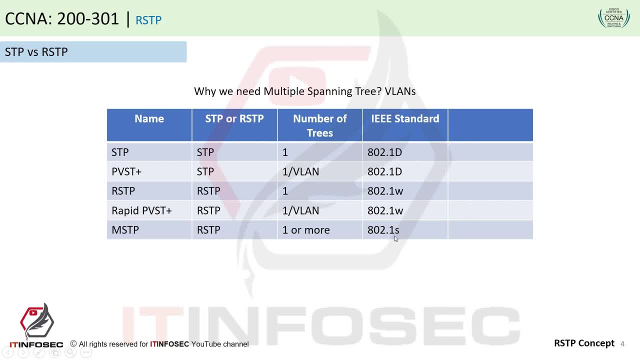 newest protocol 8 under 2.1 s. but before i i go into the next slide, let me describe more a little. rstp crate 1: 3 remind rstp crate 1: 3. it's known as cst chran withıs cst. it doesn't matter the how many number of vlans. 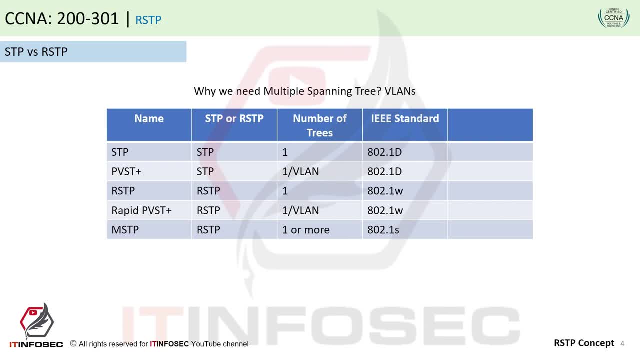 present. while RPVST Plus sends one set of messages per VLAN RSTP and RPVST Plus Rapid per VLAN. Spline 3 Plus use different destination methods for sending Hello BPDUs. Both of them are multicast addresses. One of them is a multicast address that started with: 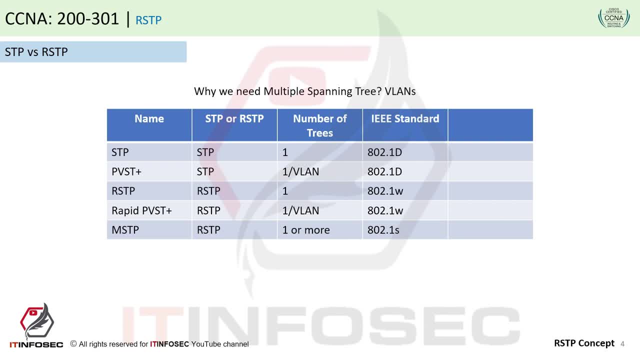 0180 and another is started by 0100.. And when we have transmission message on VLAN trunk, RSTP send message in native VLAN, but RPVST Plus send each VLAN message inside its VLAN's ID. Another item is ether channel. 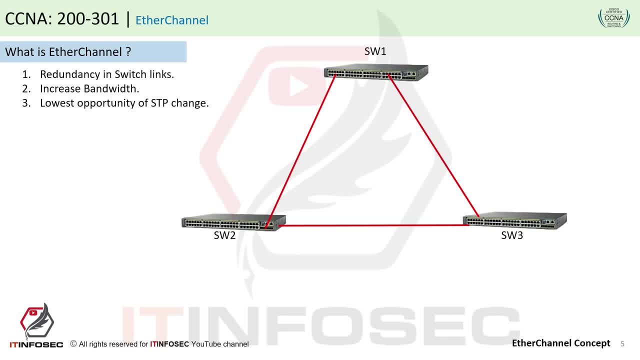 What is ether channel? Ether channel means you have configured more than one physical port between two switches or between some switches up to 8. And use all of them as one single port. But what is the ether channel benefit If you some switches started with more than one physical port and categorize all as one? 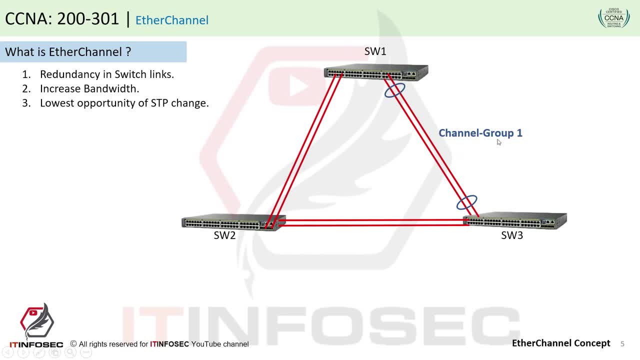 port and known as one number or known as one group, all ports known as one group, for example channel group one, channel group two or any numbers. uh, it's some. it has some benefits, for example, first is redundancy between switch, switches, links, if, if you have just one port between two switch. 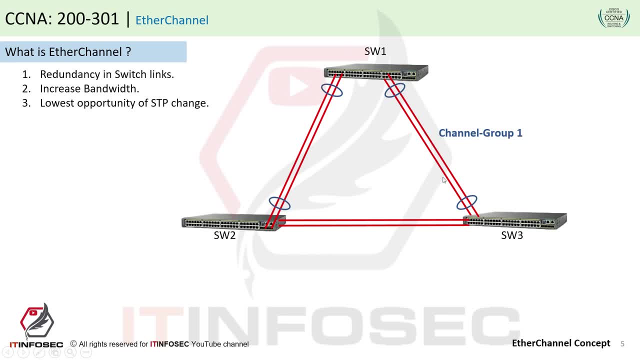 and if that port fails, the connection will be lost and disconnected and the transfer between the switches with fails. but if you have more than one physical port and all ports connected as one single port, it will provide redundancy and if one link fails, another another present link will remain. 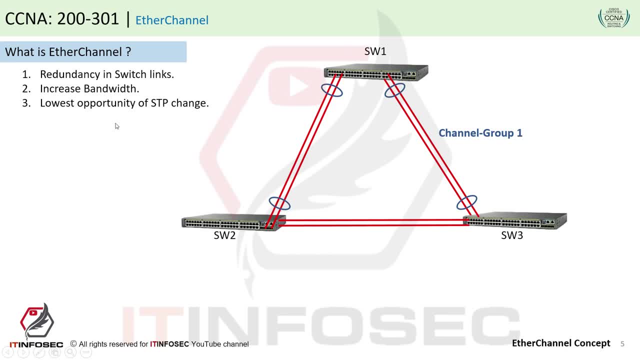 the connection between these two switches. the second benefit is increased bandwidth. if you have connected more than one ports between two switches as a single port, all, all bandwidth for all ports will be some and will provide more bandwidth or for sending traffic between them. and the third item: 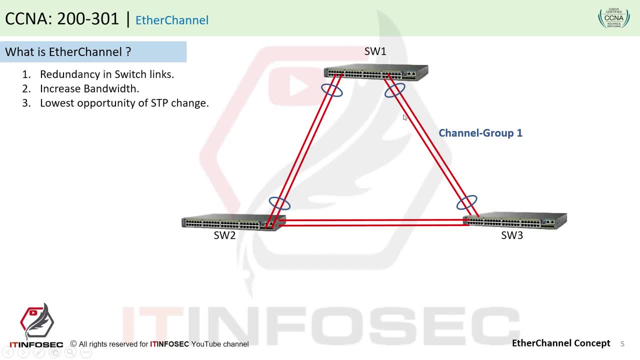 in benefits is low opportunity of STP change, just if you, if you have just one port between two switch and it fails, the STP configuration will be changed. maybe a root switch change, maybe black port will change and any other issue in STP. but if you have more than one port, the STP, the STPs, opportunity for changing port will. 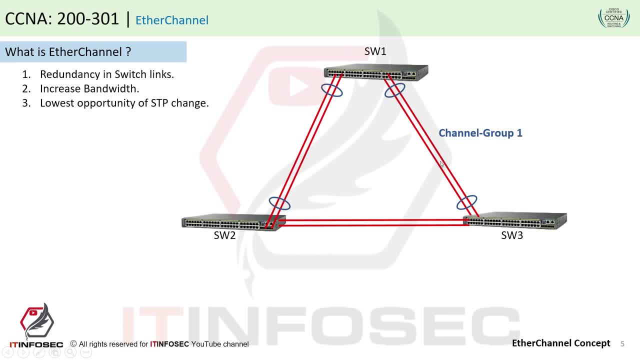 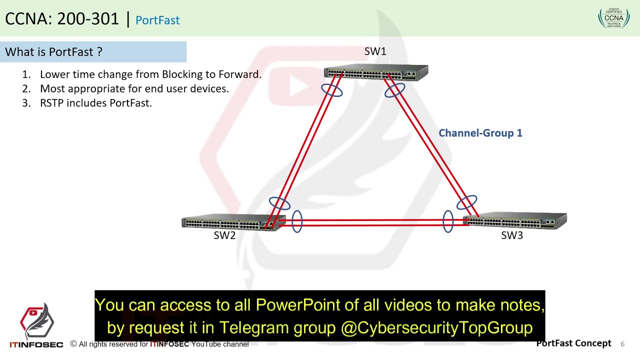 be lowest because another ports will remain. the connection between switches. okay, and what about the port fast? what is the port fast? this feature should only be configured on ports that are connected to the end-user devices. for example, if you have connected one computer to one of the ports you know on. 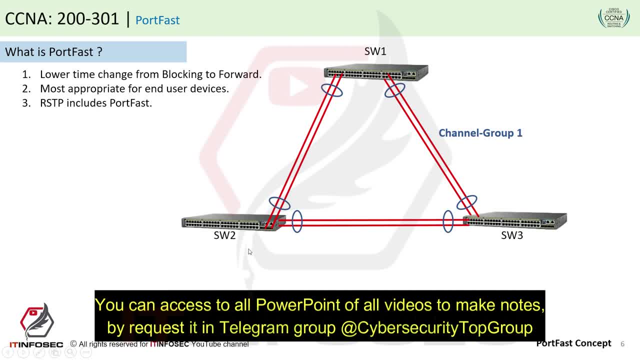 SW2. you can configure that port as port fast. you can configure that port as port fast and what does it do? I want to say simply: first it activates the port very quickly and then proceeds to learn the MAC address connected to that port. and what is? what is benefits: lower time change from blocking to forward. most. 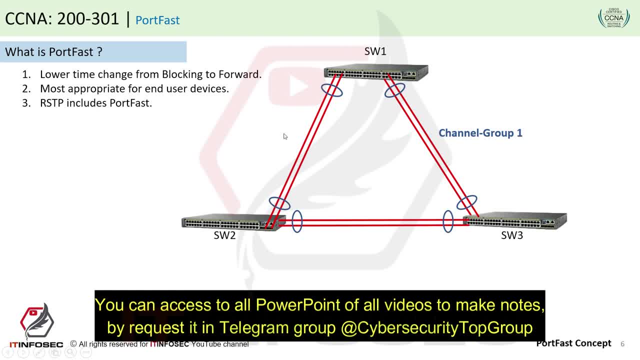 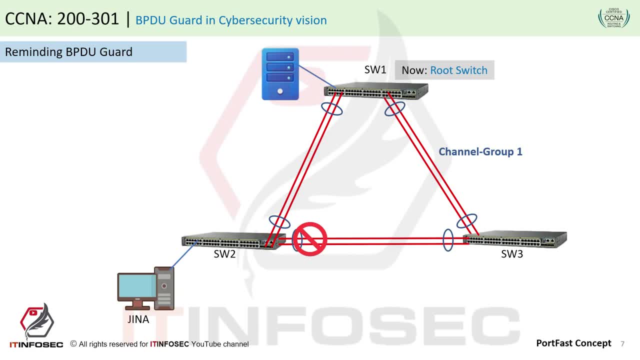 appropriate for end-user devices, and RSVP includes port fast as well. and the last item in this video is BPDU guard. the BPDU Guard feature is to prevent unwanted BPDU message from being sent by potential hackers who have gained access to the network, which I explained how to. 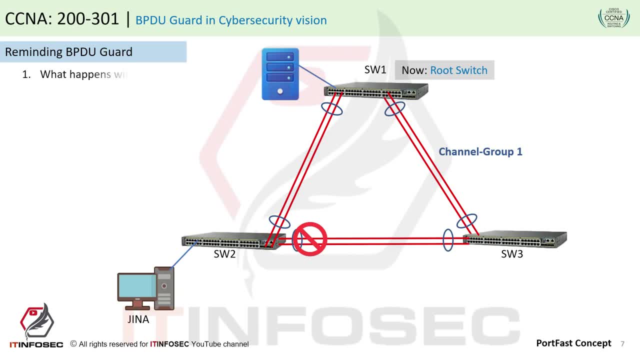 configure in previous videos. now let's see what happens if such a scenario happens and BPDU guard is not configured. imagine that we have a network in which the server is connected to a W1 and the path of sending the BPDU Guard is not configured. imagine that we have a network in which the server is. 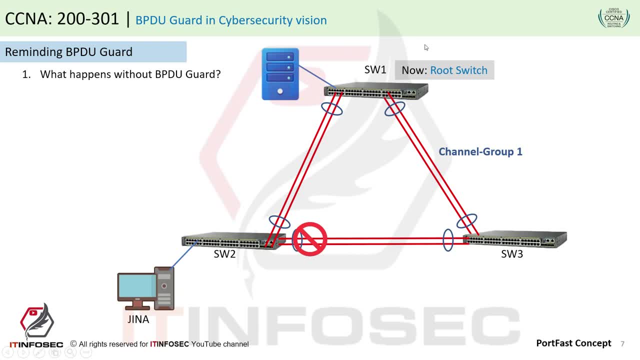 connected to a W1 and the path of sending the BPDU guard is not configured. and the path of data from the genos computer to sw2 and sw1 and the server, well, the established SCP protocol blocks the communication between sw2 and sw3. and now imagine a hacker may get, may gain, access to switch 3 or to switch. 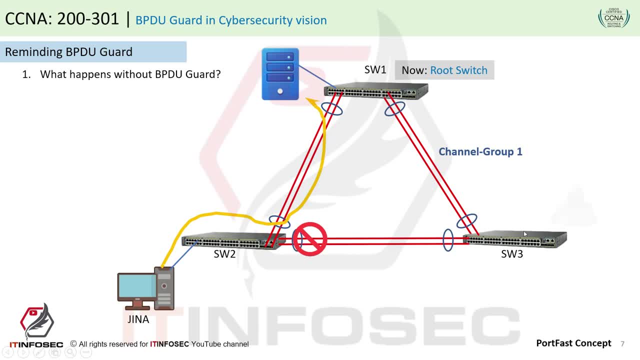 sw3. this is now. this is the path for sending data. imagine a hacker connected to sw3, but the security settings made on the switch have prevented the hacker from controlling it. but he was able to connect to one of the ports and now the system may configure itself as a BPDO issuer as a switch in, in effect, as